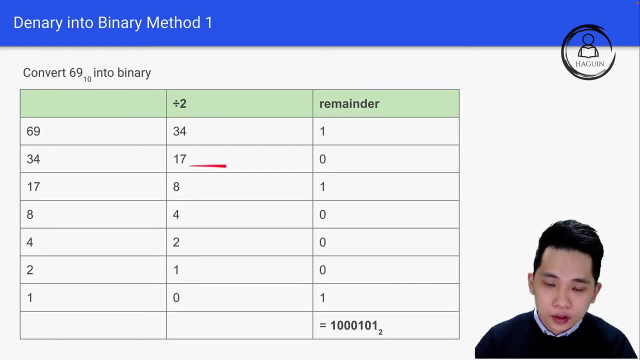 And you use 34, you move to the next row. 34 divided by 2, you get 17 as 0 as a remainder. 17 divided by 2, you get 8, and then you get 1 as a remainder. 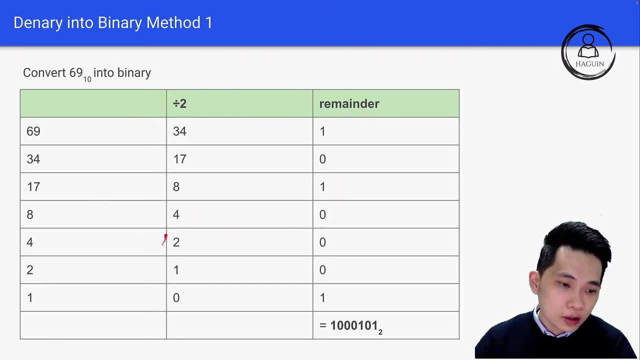 8 divided by 2, you get 4 as the answer and 0 as a remainder. 4 divided by 2, you get 2, 0 as a remainder. 2 divided by 2, you get 1 as the answer and 0 as a remainder. 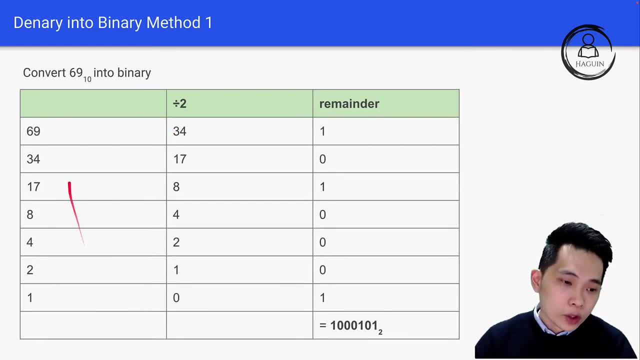 And 1 divided by 2, you get 0 as the answer and 1 as a remainder. So you actually stop when you reach 1 on the last row. And how you can actually form this number is that you actually read from the bottom to the top. 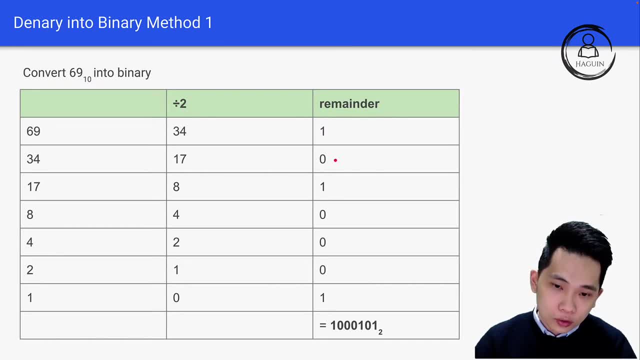 So it would be 1, 0, 0, 0.. 1, 0, 1.. So this is the final answer. So it means that 69 actually can be represented by 1, 0, 0, 0, 1, 0, 1 in terms of binary form here. 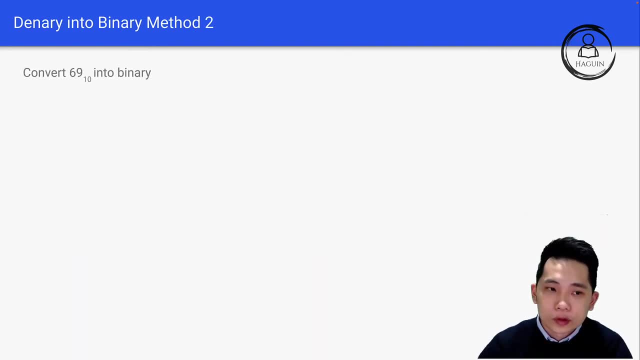 So let's look into binary using method 2.. So, first of all, how do you convert 69 into binary here? So, first of all, we have 1,, 2,, 4,, 8,, 16,, 32,, 64,, 1, 2, 8.. 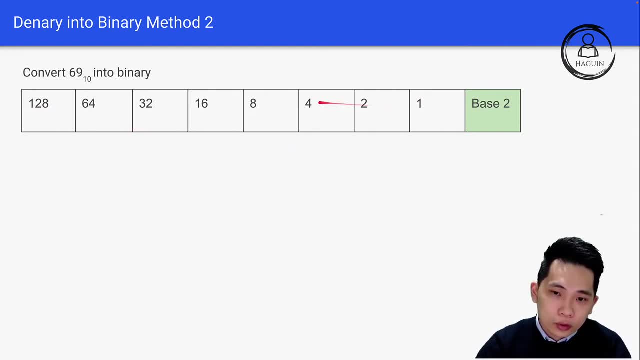 It means that all this is the power of 2 to the power of 0,, 1,, 2,, 3,, 4,, 5,, 6,, 7.. And definitely, what we're going to do is that we're just going to use some logic. 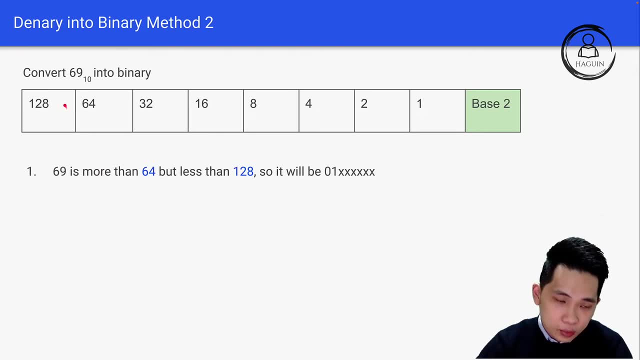 So, first of all, we know that 69 is actually more than 64. It means that 69 is between 1,, 2, and 64.. So for the bit which actually represents 1,, 2,, 8,, we'll put 0 here. 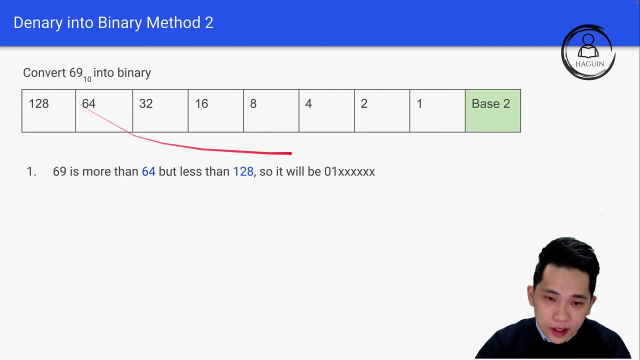 And we'll put 1 for 64.. It means that 69 actually stands for 0,, 1, and x, x, x, x, x x. And let's look at the next step. So we will use 69 minus 64.. 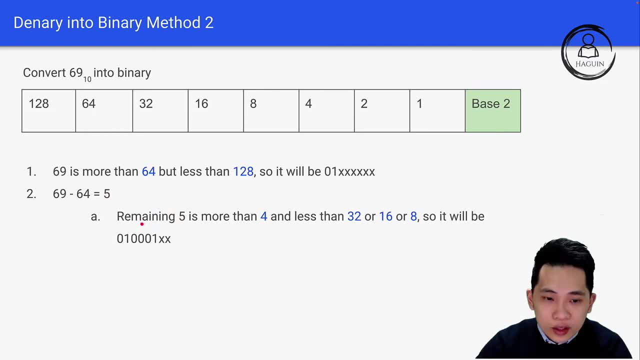 We get 5 here. So what does 5 mean? 5 means that the remaining 5 is actually more than 4.. It means that it's actually somewhere here And less than 32, or 16 or 8.. So it will be 0, 1, 0, 0, 1, x, x. 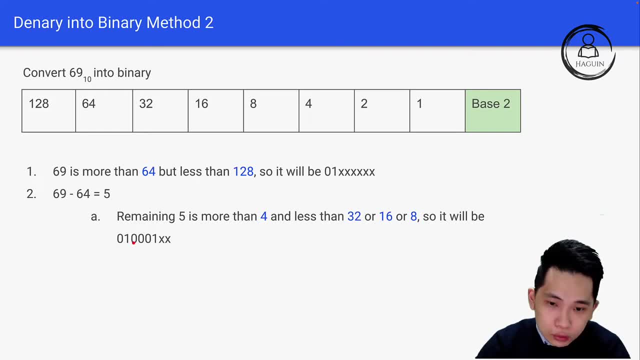 It means that for the numbers that actually represent either 32,, 16, or 8,, all will be 0. And for the one that represents 4, it will be 1. here, And we left it 5 minus 4, which is equal to 1.. 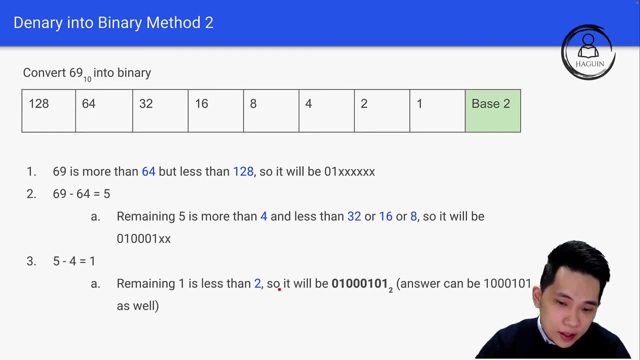 So it means that the remaining 1 is actually less than 2.. It means that, so the final answer will be 0, 1, 0, 0, 0, 1.. Since it's less than 2, it means that this will be 0. 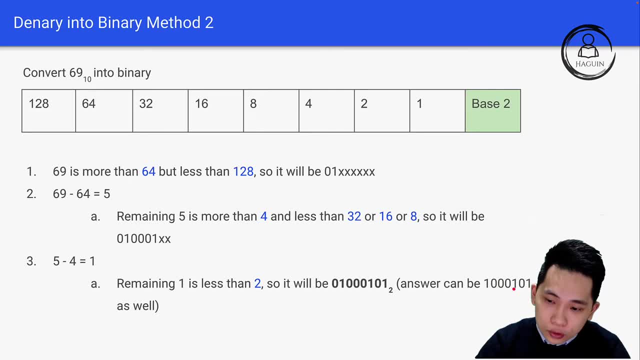 And this will be 1.. Definitely, answer can be 1, 0, 0, 0, 1, 0, 1 as well, Depending whether you want to put an extra 0 on the last bit. It doesn't really matter. 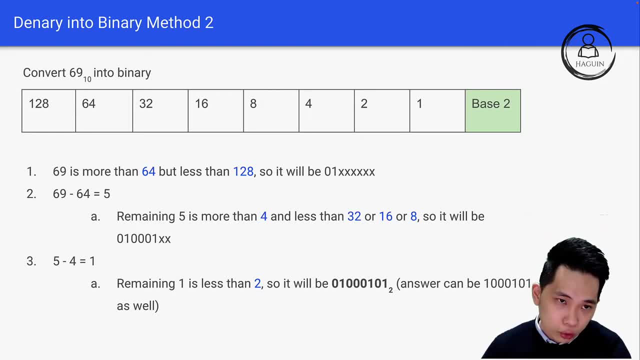 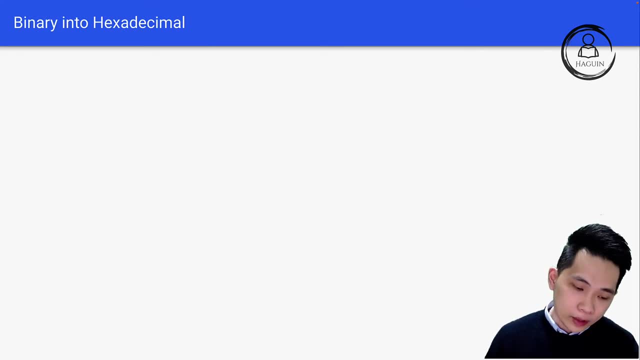 So this is what. This is the method that I actually use when I actually convert binary to binary. I personally actually prefer method 2 compared to method 1 here, So let's look into how can we convert binary into hexadecimal. So first of all, we just need to convert these 0,, 1,, 0,. 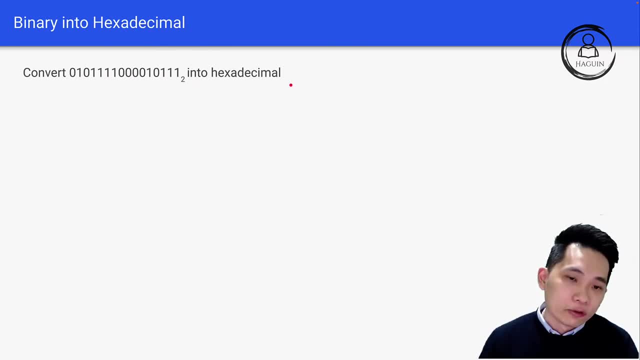 and a lot of 1 and 0 into hexadecimal. Definitely, on the first side it will look a bit complicated, But once you know the trick it's actually quite simple. So this is the trick. So, first of all, we will split into chunks of 4 bits, starting from the most right to left. 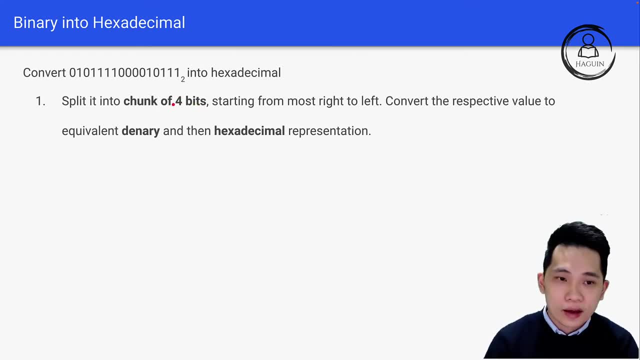 It means that you must always split from the right and then slowly to the left, So we will convert the respective value to equivalent binary and then hexadecimal representation. What it means: that for example, here we will split into 0, 1, 1, 1 as one chunk, and then 0, 0, 1 as one chunk, and etc. 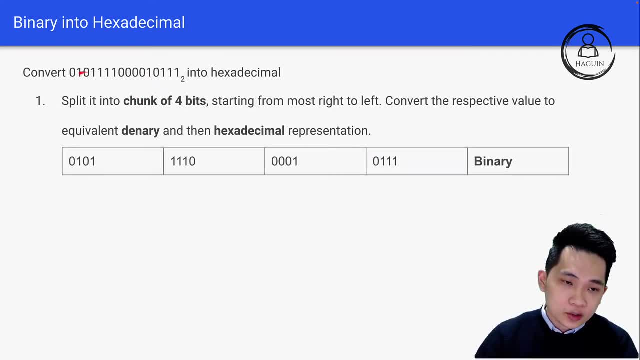 So let's look into that example. So first of all, this is what we have on the top, and then we're going to split into chunks of 4 bits. So there's 0, 1, 1, 1, 0, 0, 1, 1, 1, 1, 0 and 0, 1, 0, 1.. 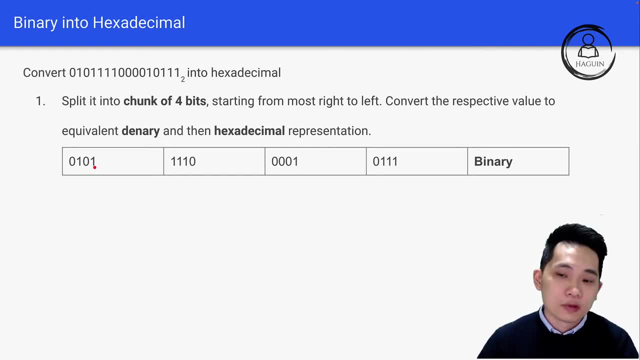 And let's look into what do they represent in terms of binary. So we definitely have a reference here which is 1, 2, 4, 8 here. And then let's say: I convert this into binary, So 0, 1, 1, 1 stands for 7, because it's 1 plus 2 plus 4 is actually equal to 7.. 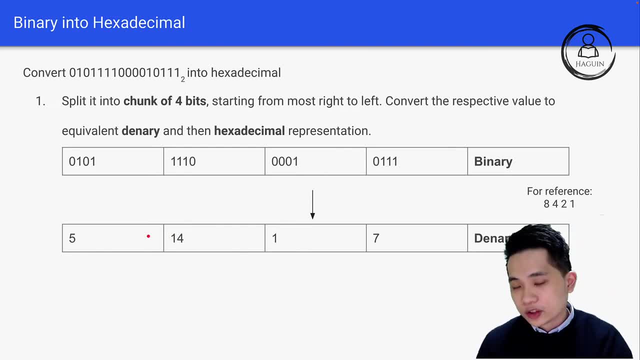 And this 1 is 14 and 5 is 5.. And the next step I'm going to do is I'm just going to convert into hexadecimal. So it's going to be 1, 7 stands for 7, 1 stands for 1 and 14.. 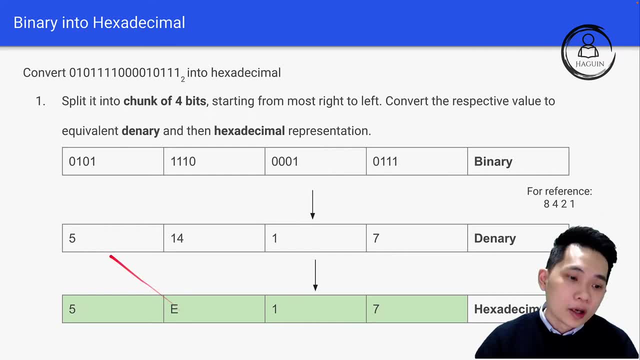 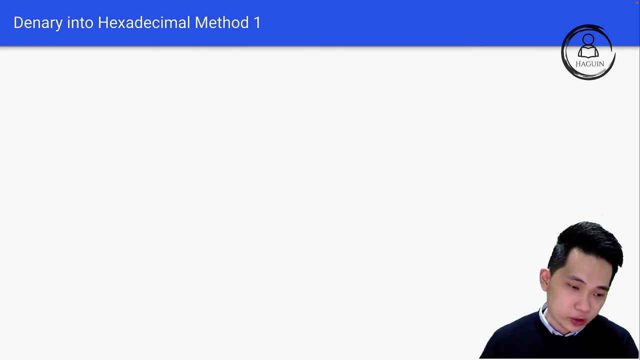 Since we only can represent single character, it means that 14 actually stands for e and then 5 actually means 5.. So this is in terms of hexadecimal form. OK. so for binary into hexadecimal we actually have two methods as well.